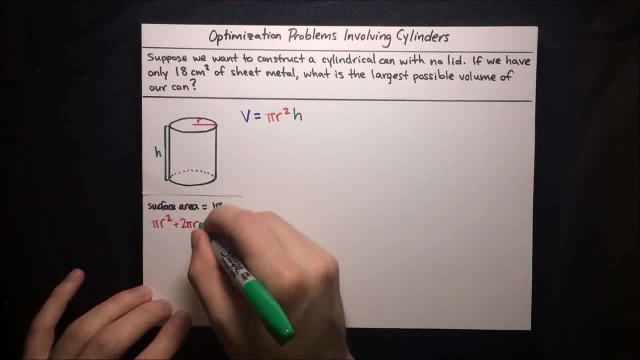 So plus two pi r times the height, h, That's got to be equal to 18.. So now why don't we solve for h in terms of r? h, because it just appears once in the equation, doesn't have any exponents. so it'll be simple to. 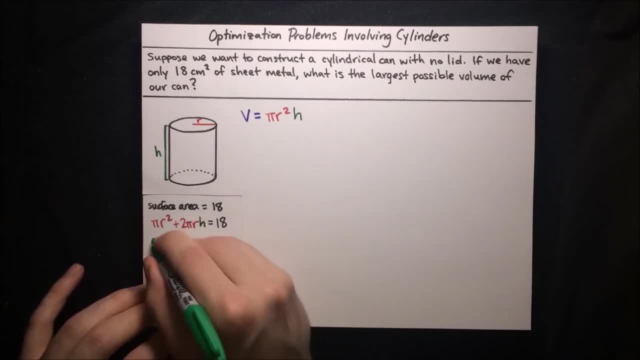 solve. First we'll subtract off that pi r squared So we'll get 2 pi r. h equals 18 minus pi r squared. and then divide by 2 pi r, You get h equals 18 minus pi r squared, all over 2 pi r. We can go ahead and sub that into our volume formula. 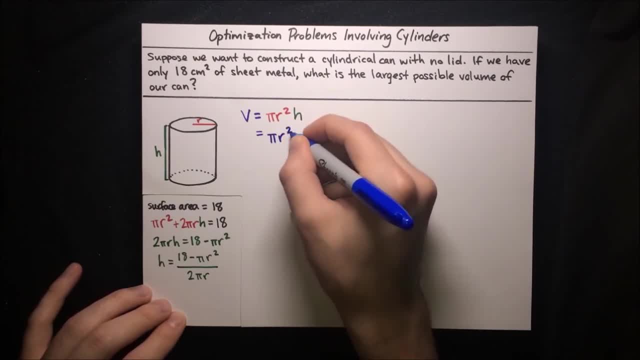 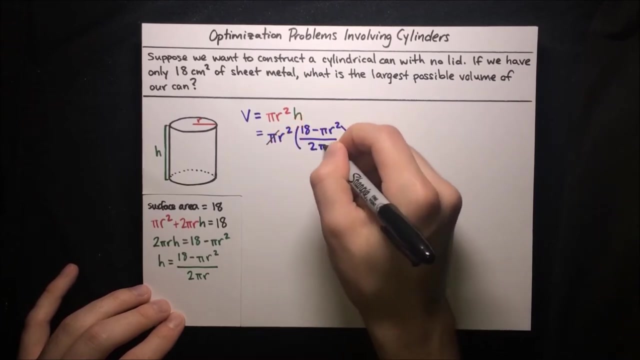 So volume is equal to pi r squared times h, and our expression for h is 18 minus pi r squared all over 2 pi r. We see that there are some things that cancel here. First of all there's pi and then the pi in the denominator, and then there's 24 plus 18 minus pi r squared. Those are all of our Fachons' errors here, All of our collaborative similarities between pi and h. give a respondents' answers when they're asked, but which means h. 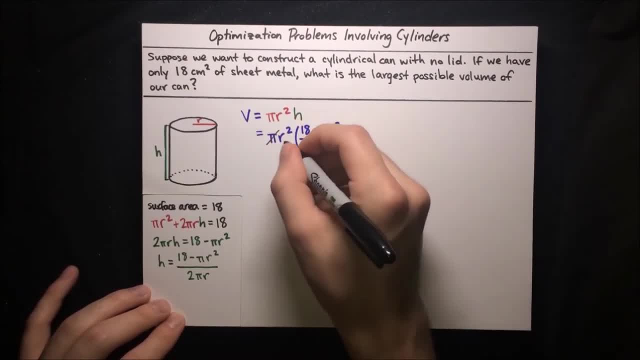 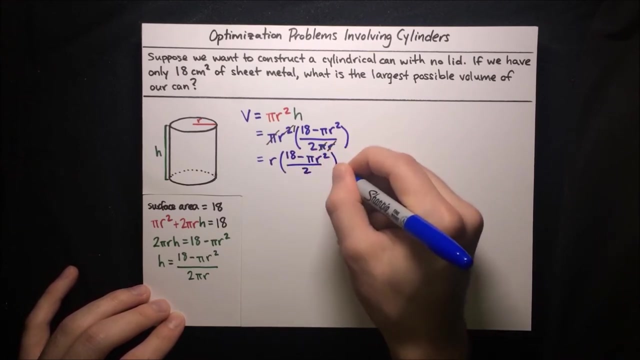 insignificant subtraction comprises a maximum of every number, room and arising � to h and m. Now quality신 And then this r in the denominator can cancel with one of these r's, decreasing the power from 2 to 1. So volume is equal to just r times 18 minus pi r squared over 2, which means it's equal to 18 r minus pi r cubed over 2. 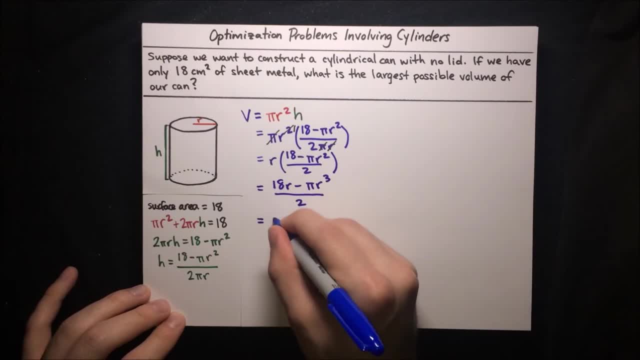 And why don't we just simplify that a little bit more? 18 over 2 is 9, so 9r. then minus 1 half pi r cubed Alright. so that's our volume function, and now we want to maximize that volume function. 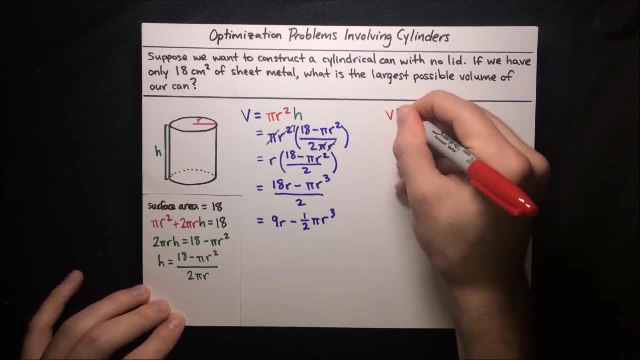 And we do that by finding the stationary points, In other words where the derivative v prime of r is equal to 0. So taking the derivative here, derivative of 9r, would just be 9.. And then, minus, applying the power rule here, bring down that exponent. 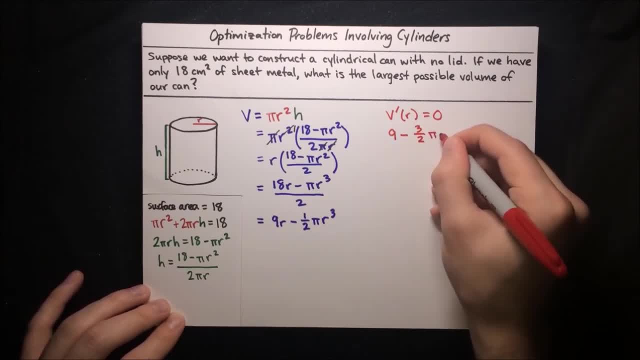 So minus Minus 3 halves pi and then decrease that exponent by 1 to get r squared. That's equal to 0, and then we just solve for r squared. So how about add 3 halves pi r squared to both sides. get 9 equals 3 halves pi r squared. 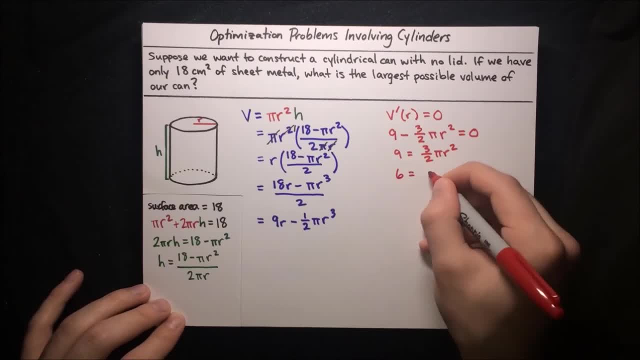 Multiply both sides by 2 thirds to get 6 equals pi r squared. Divide by pi to get 6 over pi equals r squared and take the square root. Square root of 6 over pi equals r, Positive square root because r is a physical quantity. 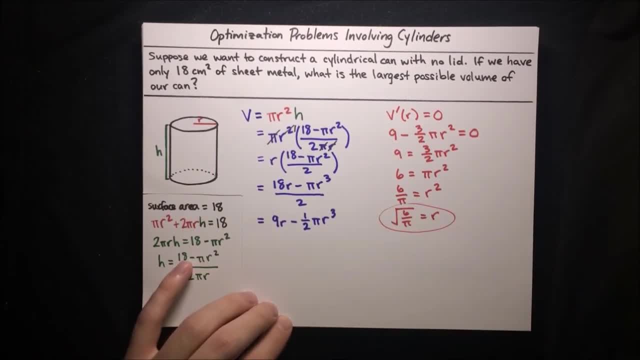 So this is our stationary point here. And why don't we verify that this is indeed a maximum of the volume function? So we'll do that using the second derivative test. Take the second derivative v double prime of r. When we do that, the constant 9 just goes away. 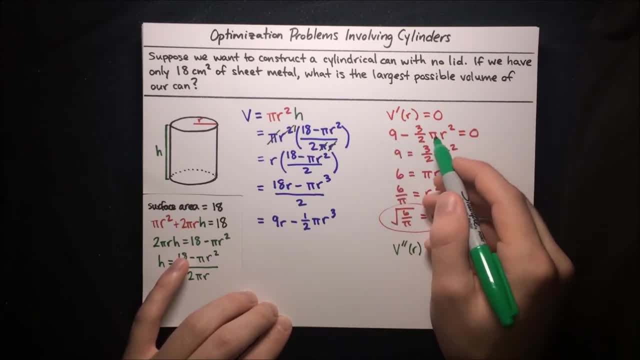 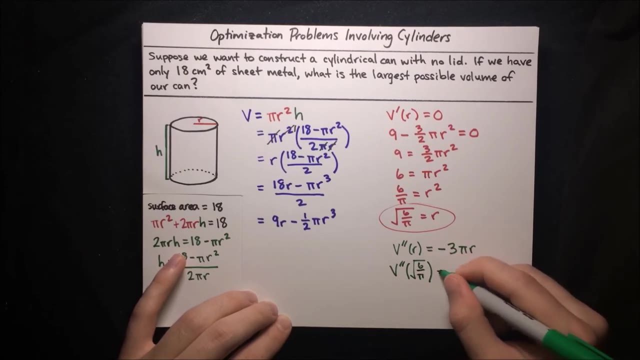 Do the power rule on this r squared That becomes 2r and then times that negative 3 halves pi, we just get negative 3. Pi r- So that means the volume. second derivative at r equals root of 6 over pi- is going to be negative 3 pi times the root of 6 over pi. 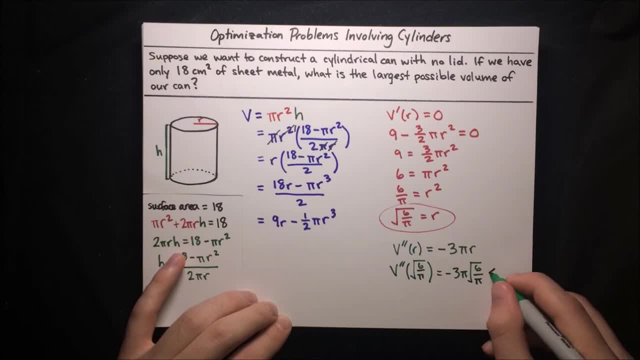 We could simplify that, but really all that matters is that's negative. And if the second derivative is negative, that means the function is concave down in the neighborhood where r is root of 6 over pi. So that means we are indeed at a negative. 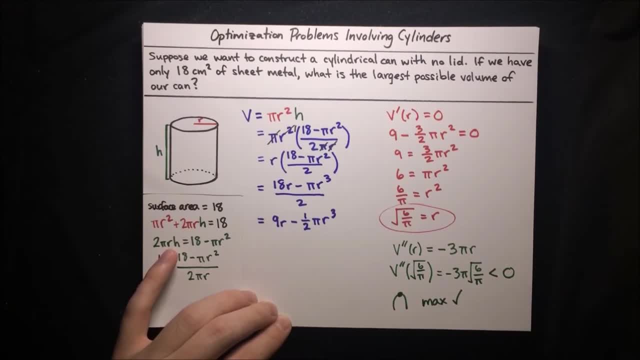 So that means we are indeed at a negative. Great. so we found the value of r, which yields a maximum, And now we just have to actually evaluate the volume function at this value of r. So the volume function evaluated when r is root of 6 over pi is equal to 9 times the root of 6 over pi. 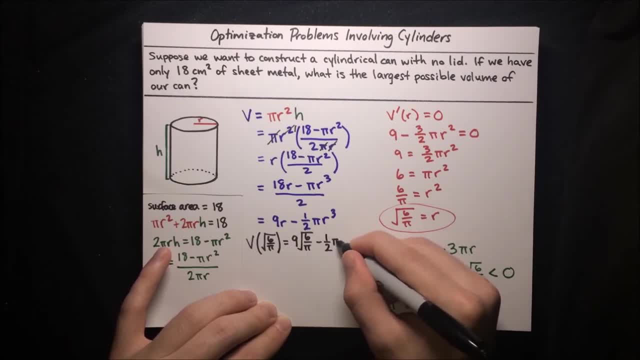 Then minus 1 half pi times the root of 6 over pi cubed, Which would make 9 times the root of 6 over pi. minus 1 half pi times, well, root 6 over pi squared makes 6 over pi. 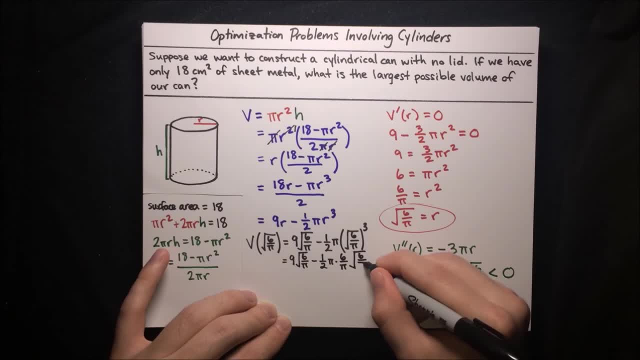 And then we still have a root 6 over pi left over And we can simplify this. This is just 9 root of 6 over pi, minus pi's cancel. And then 6 over 2 is 3, so minus 3.. 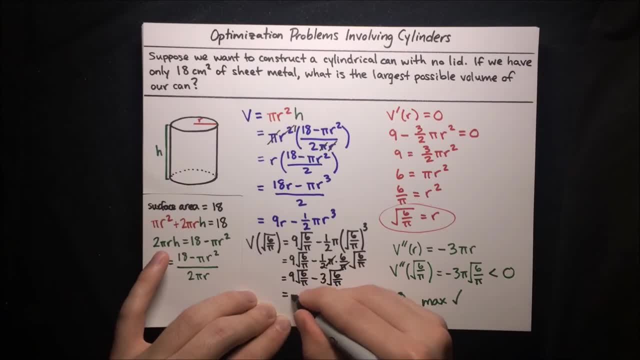 So we just have to write 3 root of 6 over pi, which makes 6 root of 6 over pi, And let's put some units on that. Units of volume are units of length cubed and length is in centimeters, so centimeters cubed. 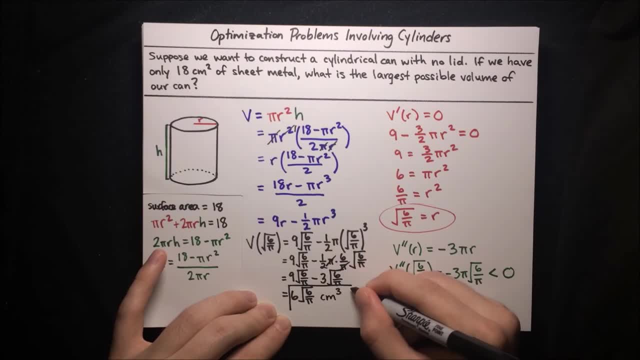 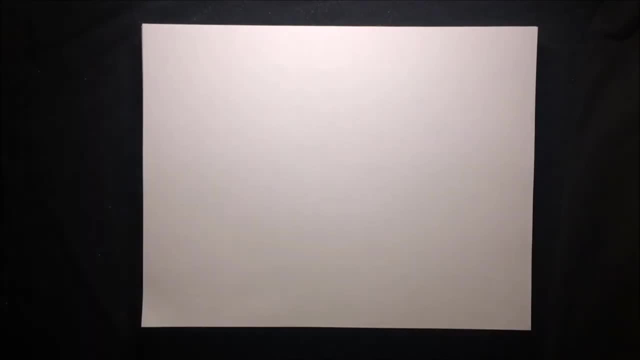 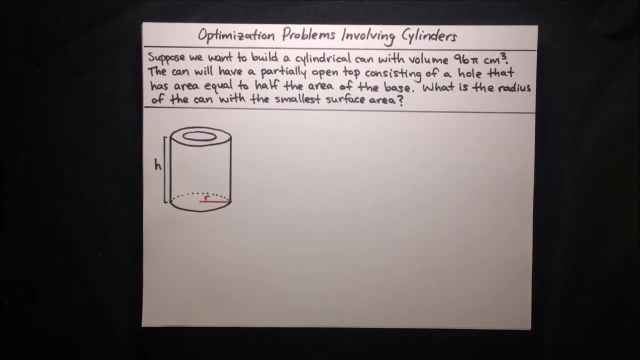 So there we go. There is the largest possible volume of our can. that is limited to 18 square centimeters of sheet metal. Here's the next problem. suppose that we want to build a cylindrical can with volume, 96 pi centimeters cubed, The can will. 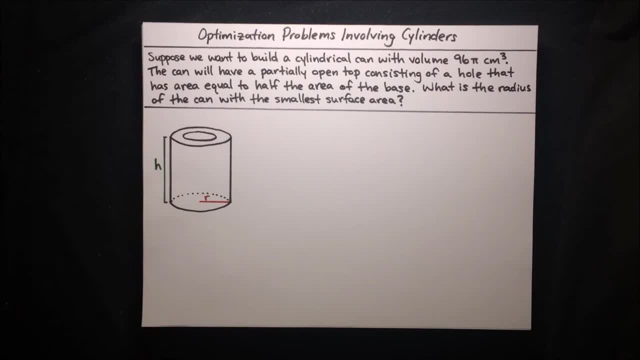 have a partially open top consisting of a hole that has area equal to half the area of the base. What is the radius of the can with the smallest surface area? Okay, so again we've got a diagram. the base has radius r, the height is h and we've got this partially open top that has kind of a. 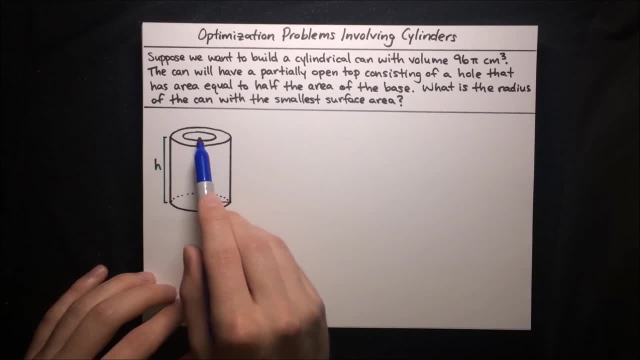 washer of material around the exterior but in the interior there is a hole and we know that hole has area equal to half the area of the base. So small circle here is half the area of the big circle there. Now we want to find what radius will minimize the surface area. So that means we need 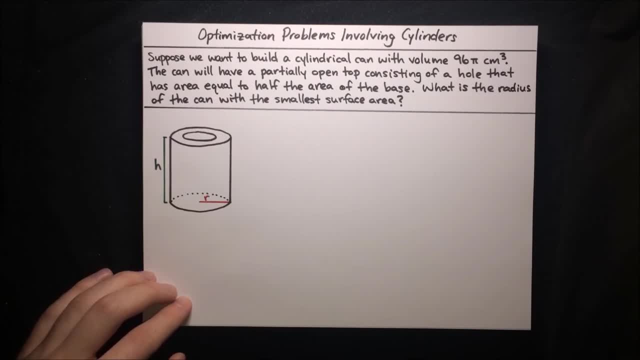 to construct a surface area function in terms of radius and then minimize that. Why don't we start by just writing a formula for the surface area? So surface area s is equal to the sum of the base area, the top area and the bottom area. So let's start by writing a formula for the surface area. 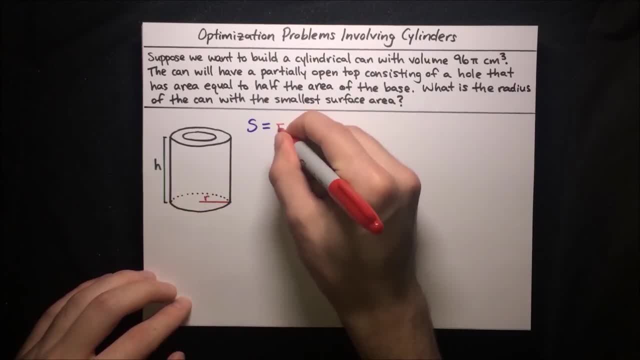 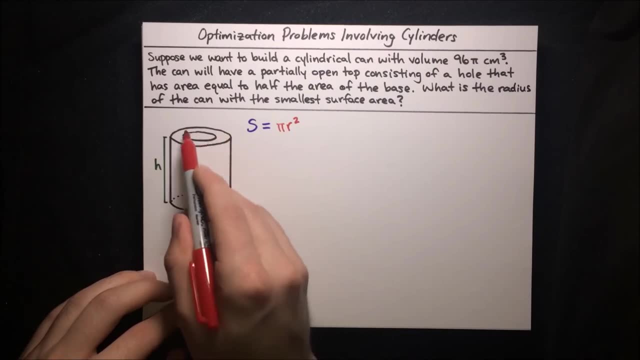 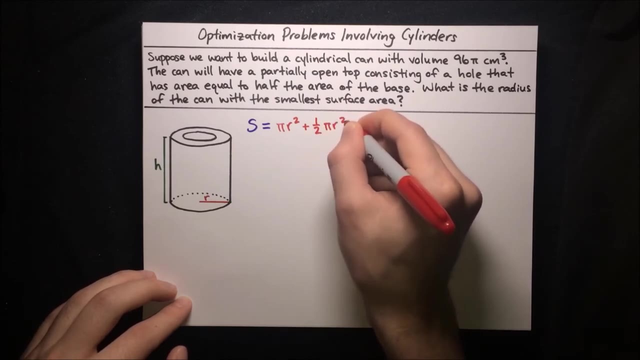 top area and the lateral area. Base area is just the area of the circle pi r squared and we know that the hole here has half that area. so the leftover washer part is also half that area. So add half the area plus one half pi r squared and then the lateral area which is equal to the 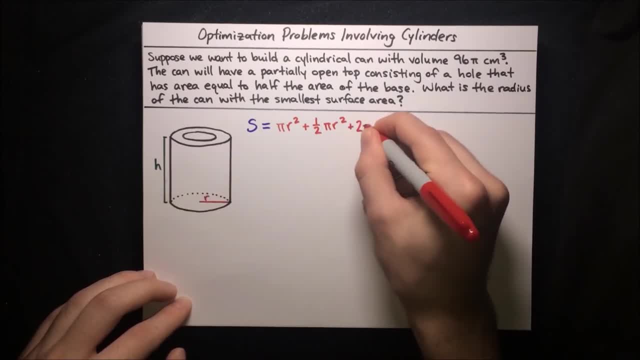 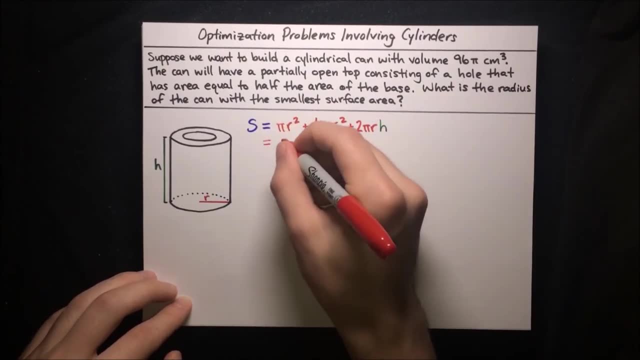 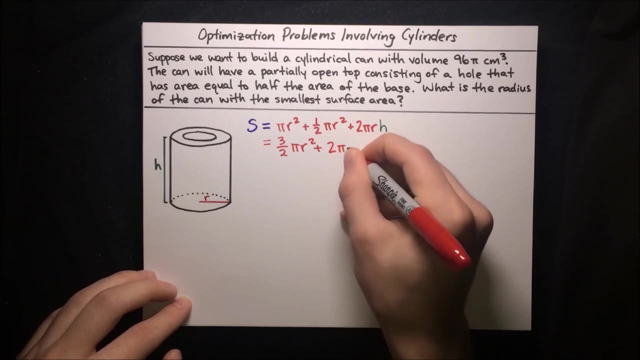 circumference times the height, So plus two pi r times h. and why don't we just simplify that a little bit? So s is equal to the circumference times the height, So plus two pi r times h, and to 3 halves pi r squared plus 2 pi r h. Now we'd like to make s a function of r, so we'd like to: 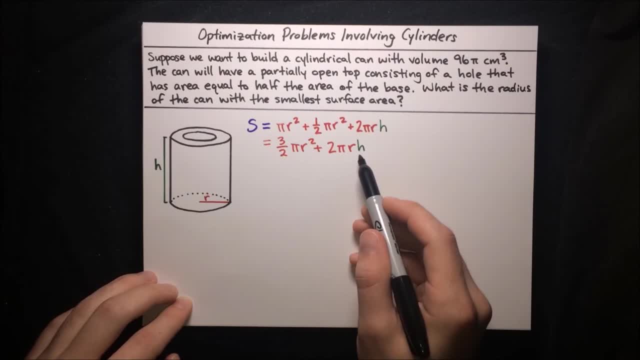 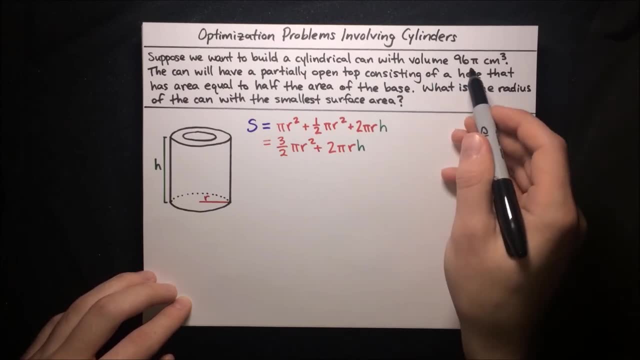 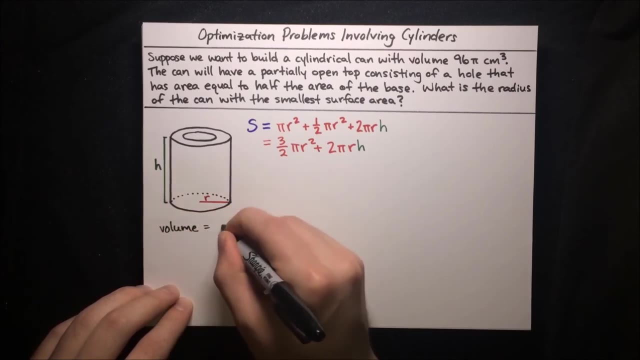 write h in terms of r, and to do that we need to figure out what is the relationship between r and h. So what other information are we given? Well, we're also told that the volume is 96 pi cubic centimeters. so we can write down an equation for that. The volume is 96 pi and we know that the 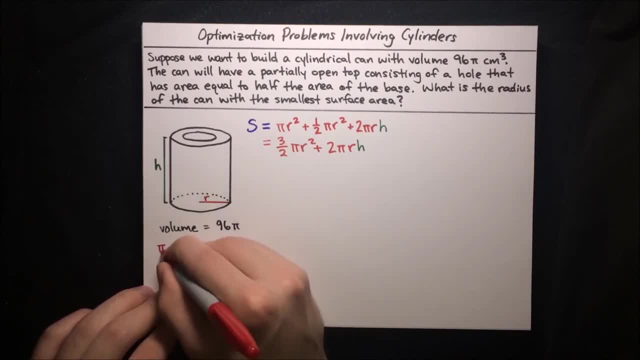 volume is just equal to the area of the base. pi r squared times the height h. So pi r squared h is equal to 96 pi and that means we can solve for h in terms of r. h is just equal to 96 pi over. 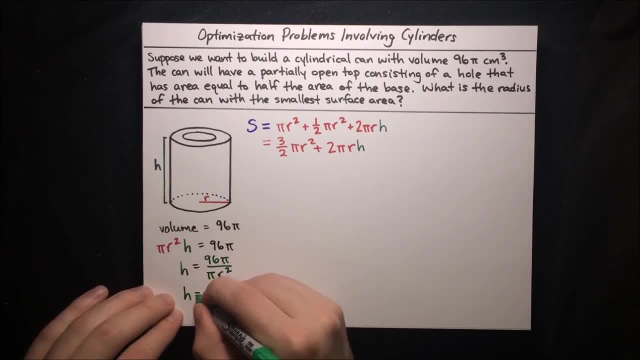 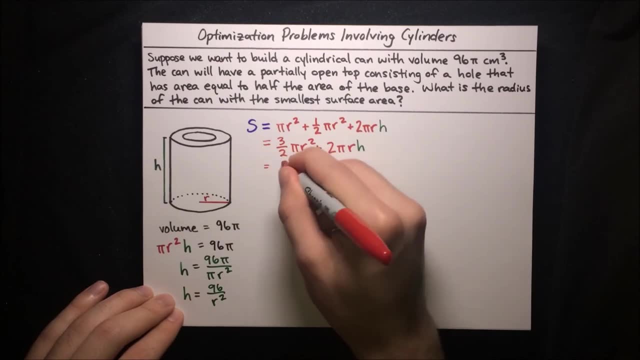 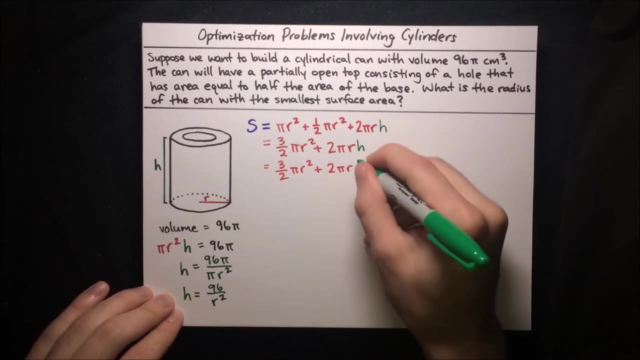 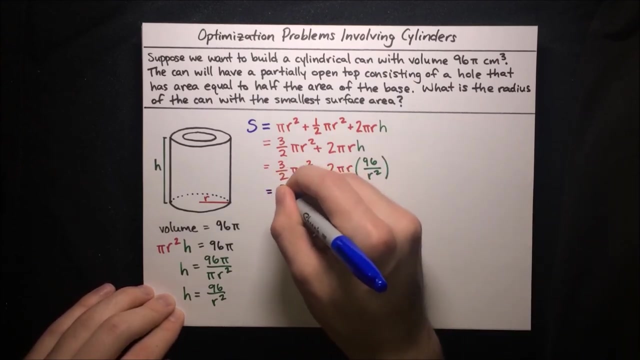 pi r squared and the pi's will cancel. so h is just equal to 96 over r squared. We can put that into our surface area function, which will now read as 3 halves pi r squared plus 2 pi r times 96 over r squared, And we can simplify this function. It's just 3 halves pi r squared plus 2 pi r. 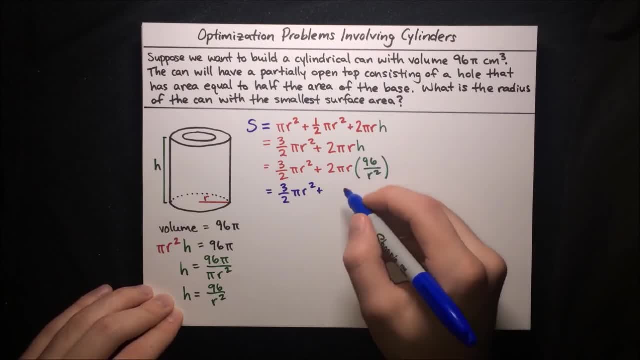 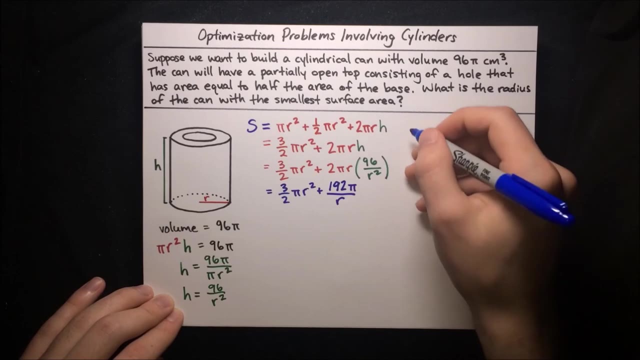 times 96 over r squared. So 2 times 96 is 192, and then we have our pi, and then r over r squared makes just over r. Now we finally got our surface area function in terms of a single variable and we can go ahead and optimize it. So that just involves finding the stationary points. 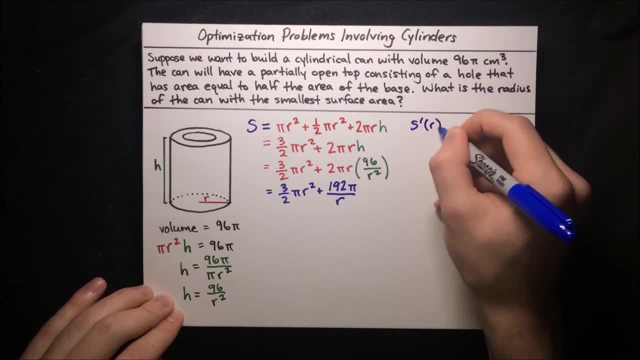 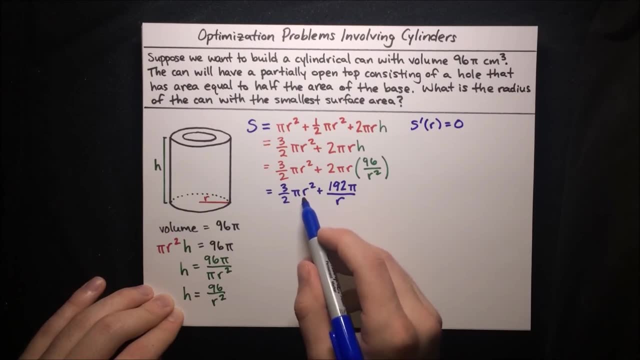 which are the points such that the derivative as prime of r is equal to 0. So taking the derivative using the power rule here on the r squared, we get 2 r squared and then that multiplies by 3, halves pi to get just 3 pi r and then 192 pi over r. 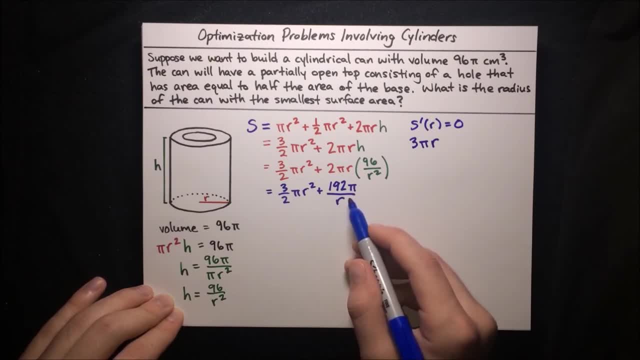 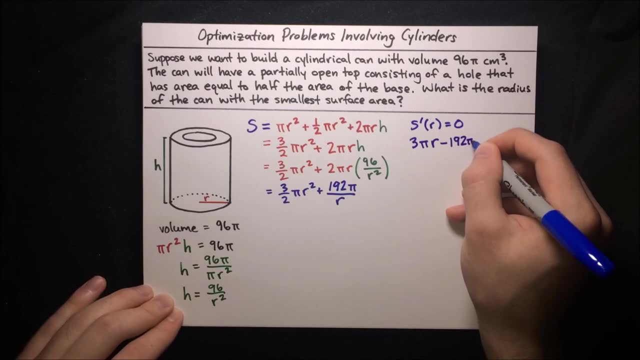 is like 192 pi times r to the power of negative 1.. So power rule brings out that negative 1, so minus 192 pi. Decrease that power by 1, so r to the negative 2, so over r squared. 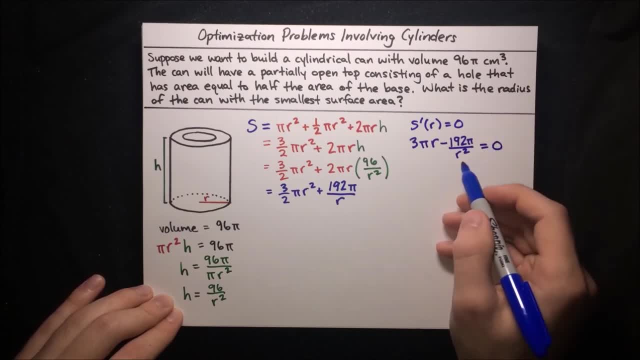 that's equal to 0.. And now to clean up this equation, since we know that r is non-zero, it's a physical equation, so we're going to have to solve for r squared over r squared. Now to clean up this equation, since we know that r is non-zero: it's a physical equation.